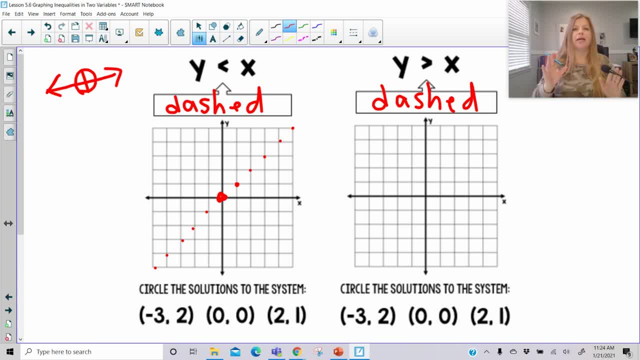 But then here's where I stop for a moment. okay, I stop and I look back at the inequality symbol And the inequality is less than which is going to tell me to make not a solid line. don't connect those points, but actually make a dashed line through them. 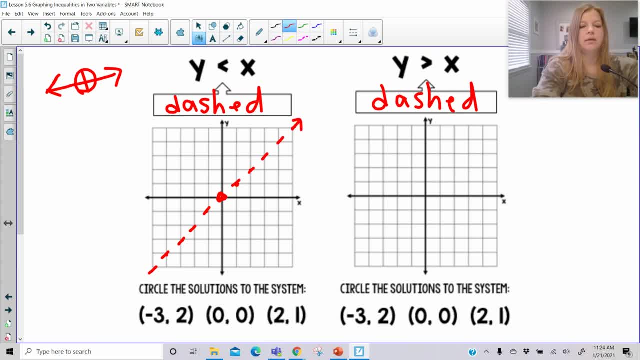 Okay, this is what this graph would actually look like. y is less than x. Now remember: if you were graphing something on a number line, you would either figure out is it an open circle or a closed circle, and then you'd have to figure out which direction to shade. 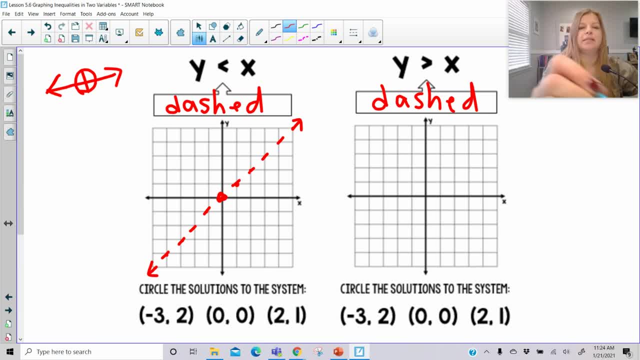 Well, this is going to be pretty simple. This says y is less than x. Okay, the inequality says y is less than. So that means we need to look at the y-axis. Where do y values get less? Do they get less at the top of the y-axis or do they get less at the bottom of the y-axis? 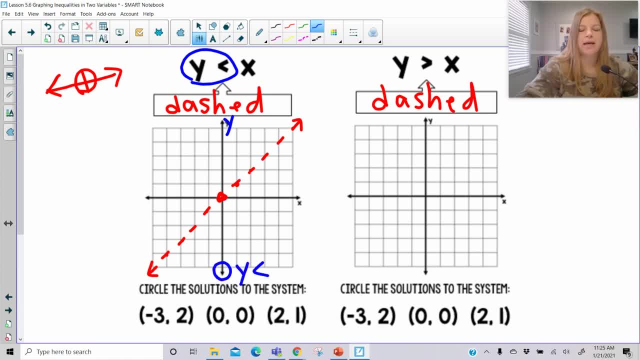 This is where y values get less. So here's what this is going to mean now. This means that instead of, like, shading on the number line, we actually go ahead and we shade in on the graph, And so look The side of the y-axis that I circled down here. 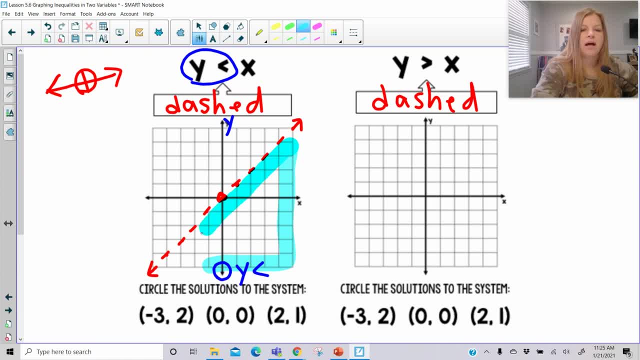 This is the entire side of that dashed line that I actually shaded all the way up to the dashed line. Now remember what an open circle would have meant on a number line. An open circle means that's where the solutions start, but that that number isn't actually part of the solution if it's in the open circle. 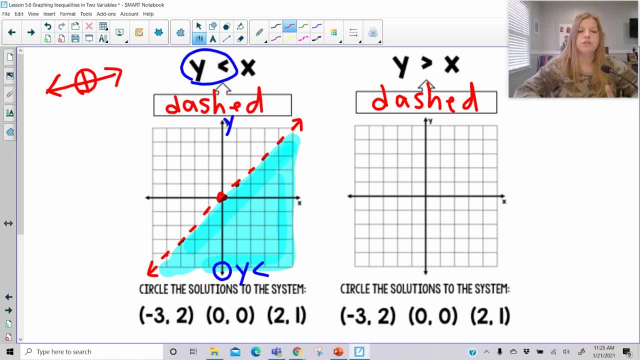 The same thing is going to apply for a dashed line. So So if I say to you, circle the solutions to the system, negative three two is up here. That's definitely not in the shaded region. So negative three two is not in the system. 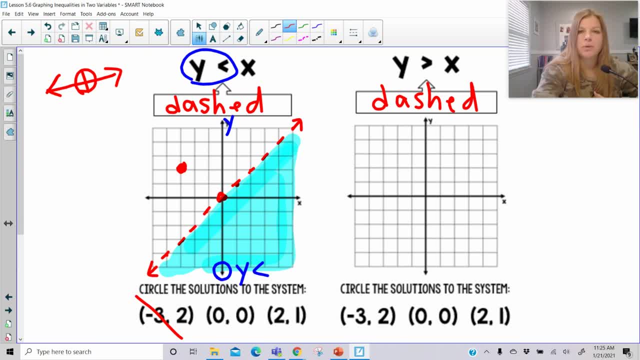 Zero, zero, zero, zero is right here at the origin and it's on the dashed line. And if something's on the dashed line, it's just like it being on the number line with the open circle. That's also not a solution. 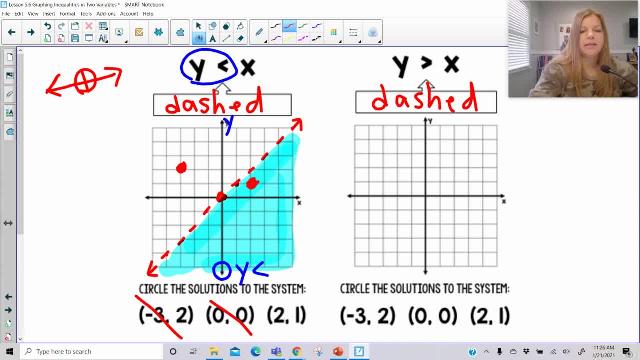 However, two one is right here and two one is Definitely in the shaded region. Let's take a look at the next one. Why is greater than X? So why is greater than X? still has a Y intercepted zero, a slope of one. 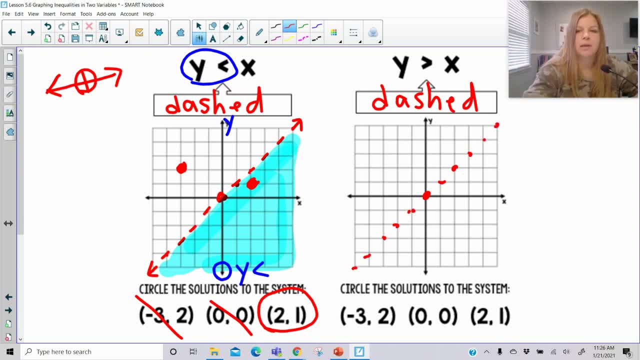 Remember. you start graphing it as if it's an equation. I stop. I look at the inequality symbol. greater than would have been an open circle on a number line, So on a coordinate plane it is still going to be a dashed line. 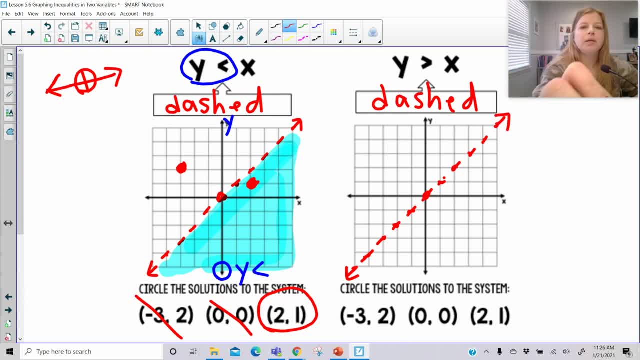 That's how we represent, like the open circle. So now I'm going to go ahead And look at the inequality. This inequality says Y is greater. So that means we look at the Y axis and we say to ourself: where does the Y axis get greater? 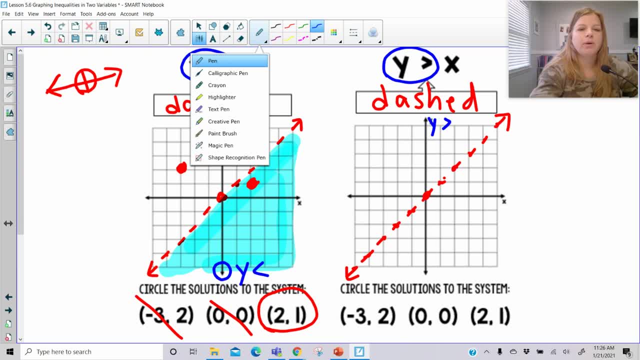 It gets greater at the top. So now, when I want to go ahead and shade in the region of all the values where Y is greater than X, This is the side of the graph that I would shade in. So whatever side I follow the inequality by wherever it says it's greater. that's the side of the graph you shade all the way. 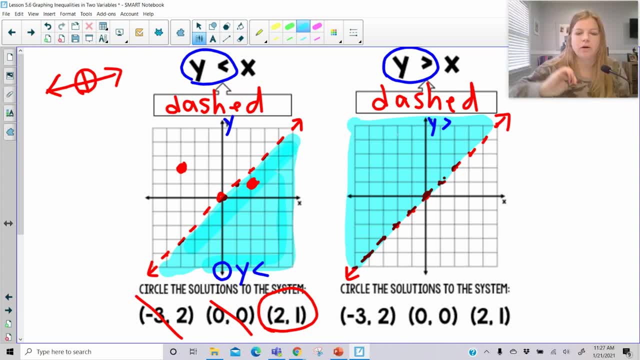 I notice I extend Through all the quadrants here all the way across that dashed line. So then, if I want to now answer negative three, two, that's definitely in the shaded region. Zero, zeroes on the dashed line, not part of the solution. 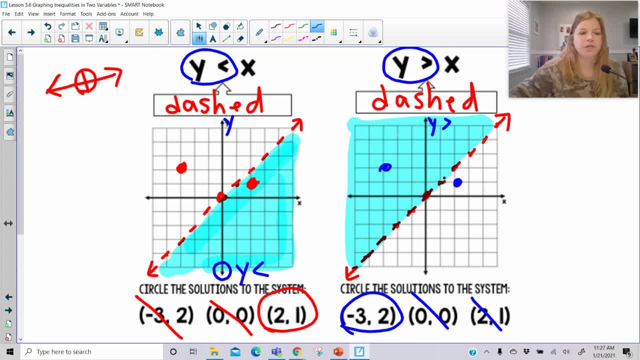 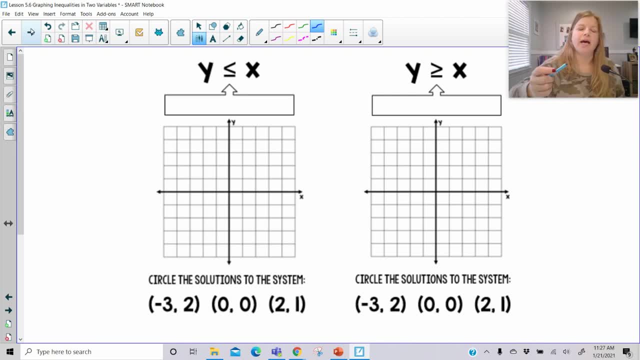 And two, one is here, Definitely not in the solution. Okay, So I hope that you felt, feel like you went along with that pretty easily. Now let's take a look at the second half of things. So now, if this was a number line and you had a, 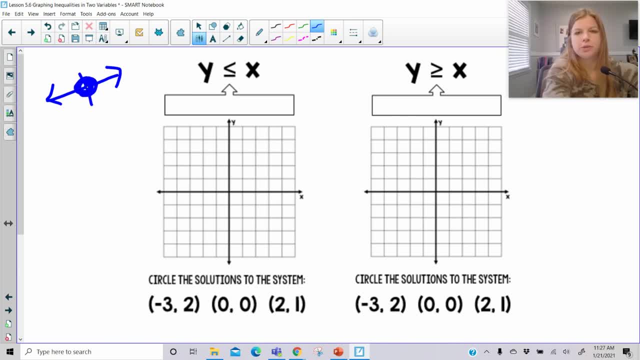 Less than or equal to symbol. we know that would have been a closed circle on a number line, which actually means it's going to just be our classic solid line. Okay, So those are the options: dashed or solid, and solid is just what we've been so used to at this whole point. 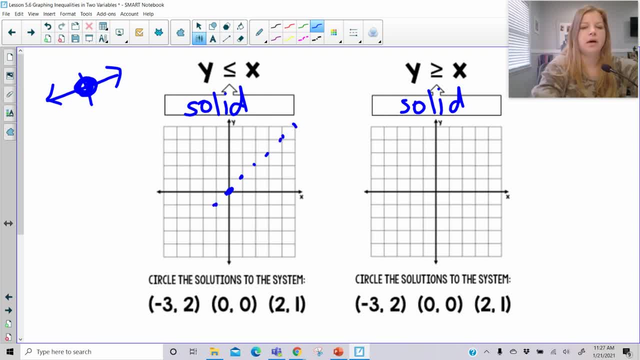 So if I go to graph this line now: um, Y, intercept of zero, slope of one, I can now connect them with a solid. And then remember, we look at the inequality. So the inequality here says Y is less than or equal. 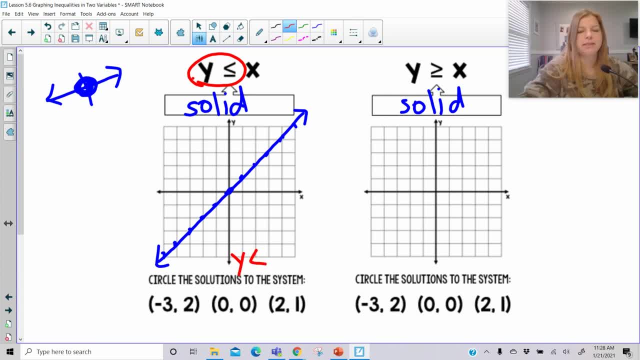 To well, down here is where Y gets less than so. that's the side of the graph that I go ahead and shade, and I shade it the whole way up until that line, because that's where Y gets less. Now, if I want to go ahead and circle the inequalities that are part of the solution, well, negative three. two is up here. 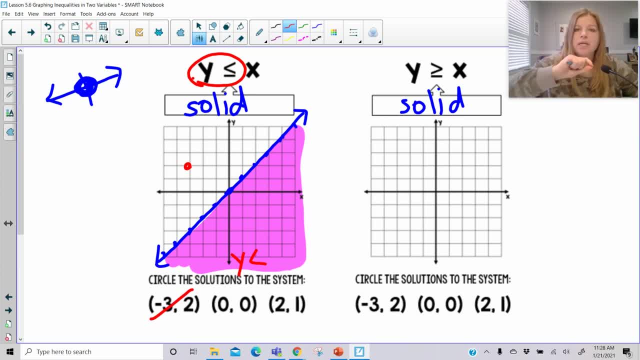 No, but now look at zero, zero, zero, zeros on the solid line. And we remember when we had A number line, If the number was in the closed circle, it was part of the solution. So now, if a point is on the solid line, it is part of the solution. 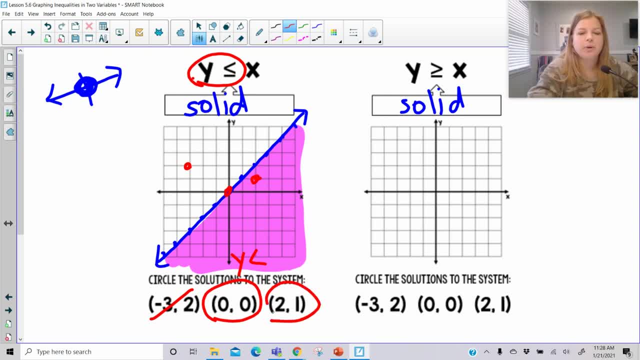 And so that's good. And then two, one is part of our solution, Awesome. So now here, Y is greater than or equal to X. So what we're noticing here, guys, is that, um, we're now realizing when we use a solid line, when we use a dashed line, 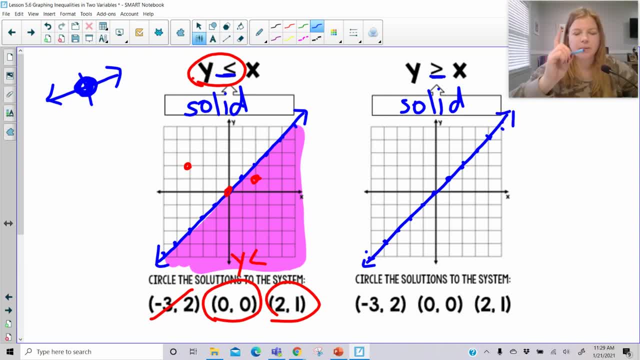 So solid is always when we have the equal to part. Okay, That's like a big um thing to look at. This is now saying Y is greater than or equal to. well up here This is where Y values get greater. So that's going to be the side of the graph that I'm going to shade in. 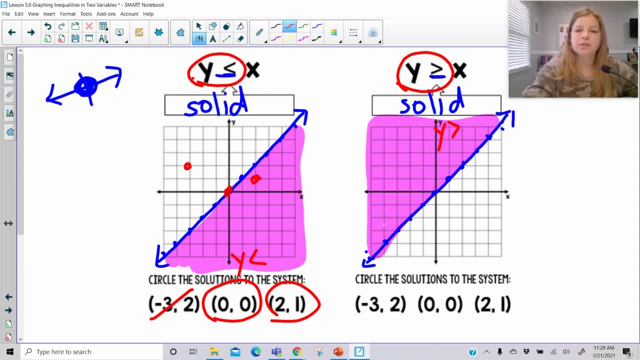 And then I'm going to go ahead and answer this question circle, the solution So negative: three, two is definitely in the solution set Zero- zero, we know, is directly on the line. And of course, two: one is not in the 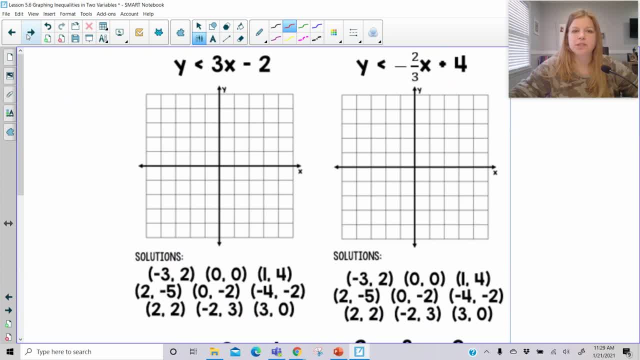 Shaded region. Okay, So now we're going to take a look at just some more inequalities. same kind of practice, just better skill, um more situations going on. So Y is less than uh three, X minus two. So I would plot a Y intercept at negative two, a slope of three. 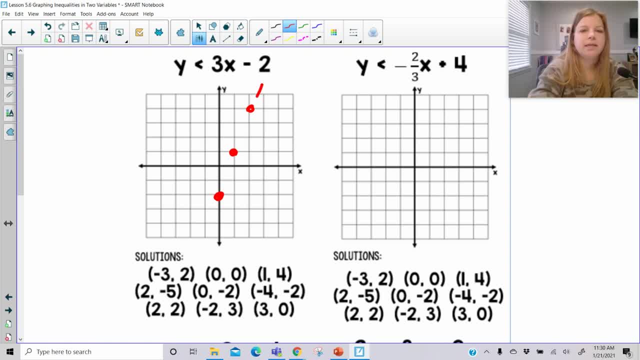 I check the inequality. It says less than less than is a dashed line. Now it says I need to shade in where Y is less than. So look at the Y axis. where does a Y axis get less as you go up or as you go down? it definitely gets less down here. 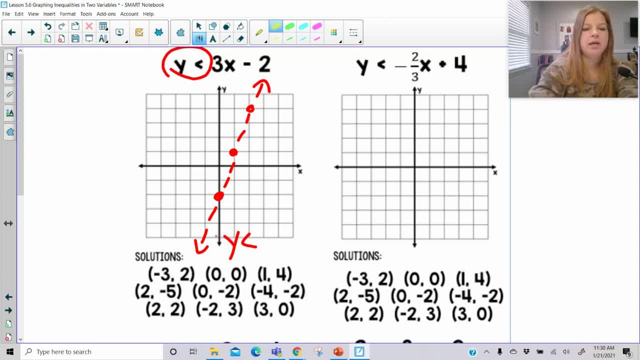 And so then that's the side of the graph I will shade. you're going to see, I'm just so consistent with my explanation on this And usually when I'm in class with my students explaining this, I feel like my success, uh, with my students and understanding this process of how to know which side to shade just really becomes so second nature. 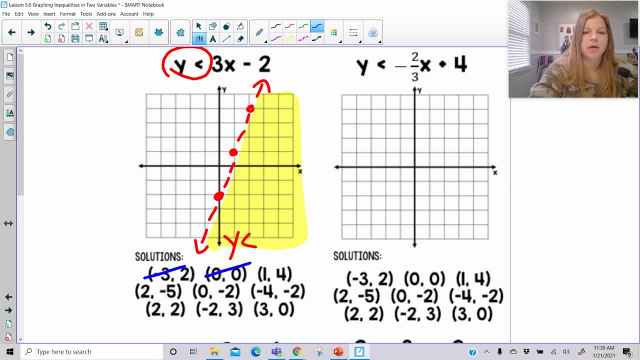 So negative three: Two, no, zero. zero no one. four, no two. negative five: Yes, this two negative five is down here. Zero negative two is actually on the dashed line. So no negative four. negative two: no two. two is here. 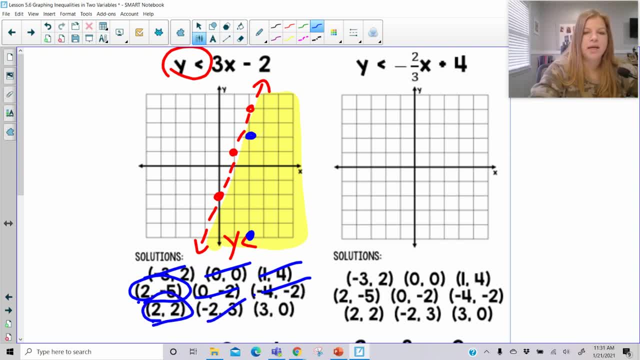 So that's good. Negative two: three definitely not. And three zero. Those are definitely in the solution. Next one: Y intercept, a positive four Slope Slope of negative two thirds. I look at the inequality: It's a less than which again means it's going to be dashed. 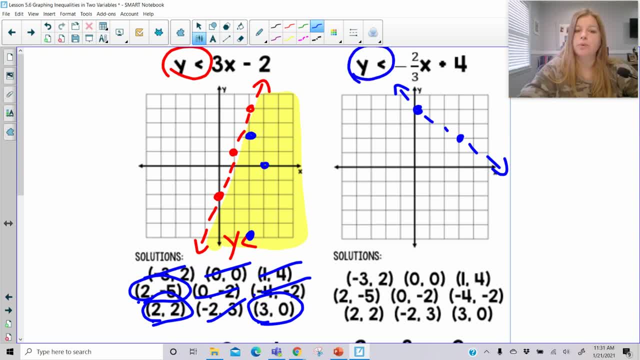 It says Y is less than So. I look at the Y axis. Where does the Y axis get less? It gets less at the bottom here. So now that is the side of this entire graph that I shade in. All of these coordinate points here are part of the solution, except for points, of course, on the dashed line. 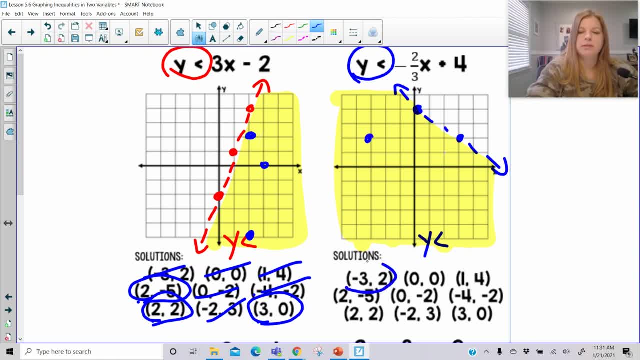 So now negative three: two is here, That's good. Zero: zero Good. One. four is up there, No good Two. negative five is good, It's down here. Zero negative two is good. Negative four: negative two is good. 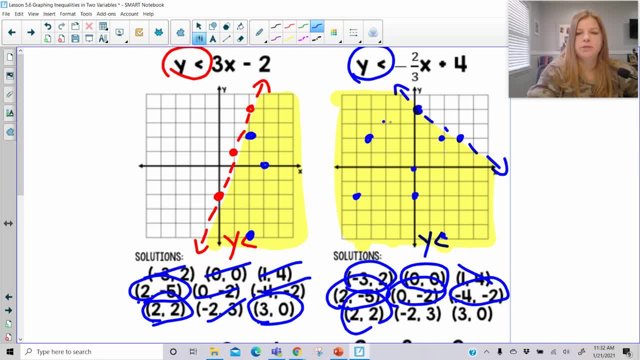 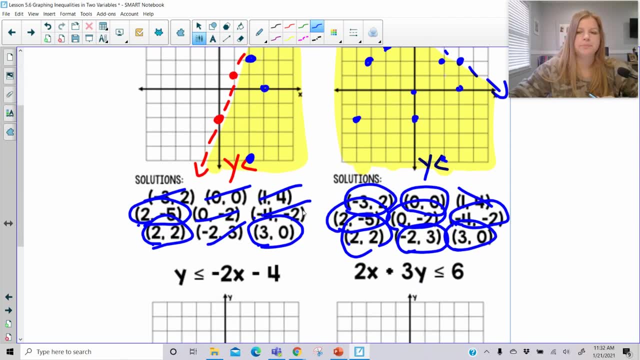 Two, two just makes it Negative. two, three is good And three, zero is good. So look, only one of those ordered pairs actually did not work. Okay, so now less than or equal to, So again we plot the Y intercept. 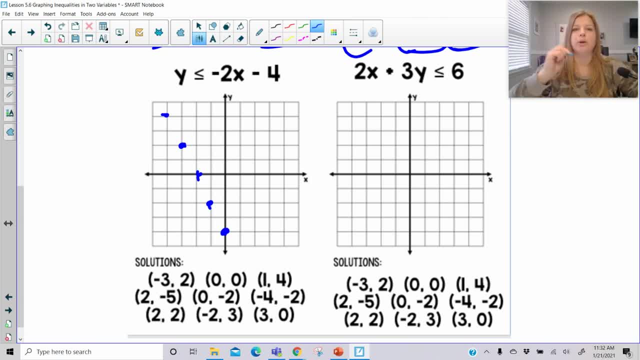 We plot our slope. But now when we look at the symbol, it's less than or equal to, So that's going to mean it's that solid line. Okay, the moment you have the equal to part of the inequality, that's when it's a solid line. 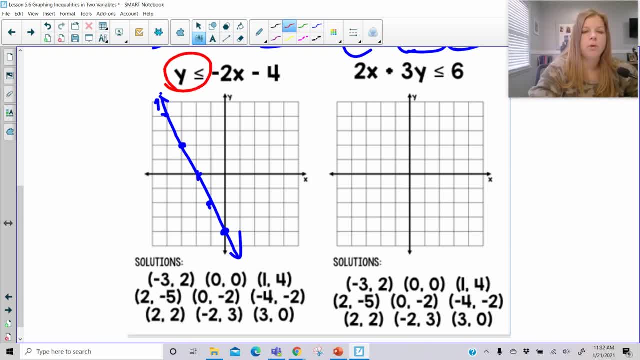 And now look at saying Y is still less than or equal. Well, Y gets less down here. Look where the arrow is. So that's the side of the graph that I would shade in And then remember if a point's on the solid line, it is going to be part of the solution. 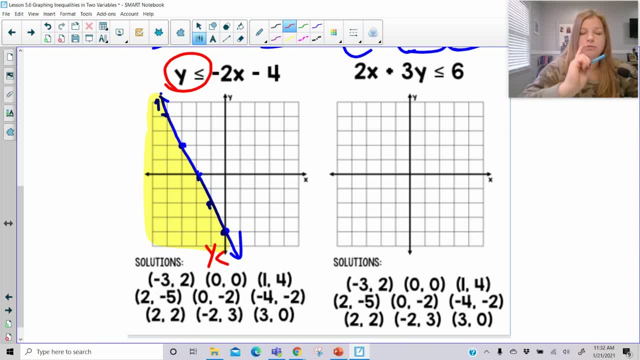 It's going to be good. So negative three, two. Look, it's right on the solid line right here, So that one's good. Zero, zero, no One. four, no Two. negative five: nope. 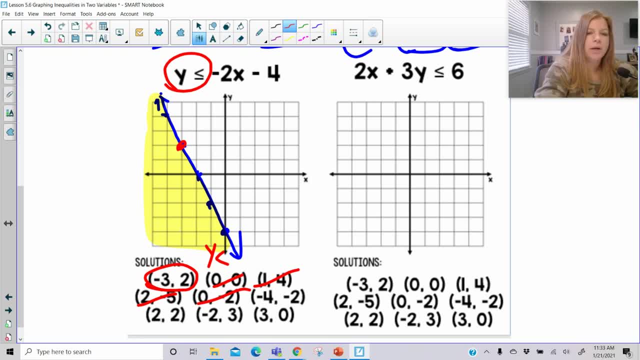 Zero negative, two no Negative, four negative. two is down here, That's good. Two, two no Negative, two, three nope And three zero Nope. Okay, this one here now. So it's in standard form. 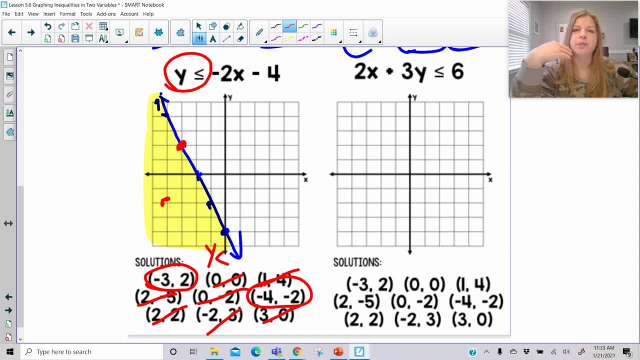 We could rearrange it, put it into slope intercept form. I personally prefer intercepts. So if I want to find the X intercept, remember that would be you cross out the three Y, So it's two. X equals six, So X is three. 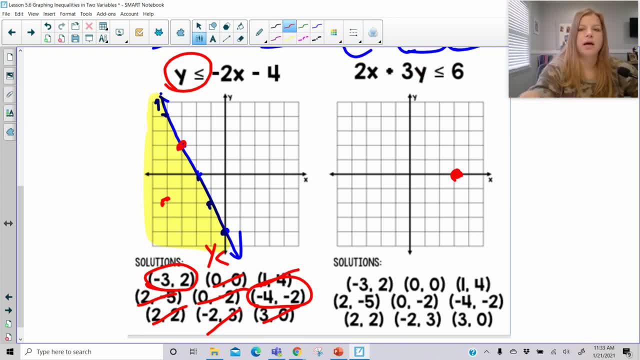 And then if I want to find the Y intercept, I would basically cross out the two X Three. Y is equal to six, So that means Y is two, And then I can see my slope is happening here. It's actually a slope of negative two thirds. 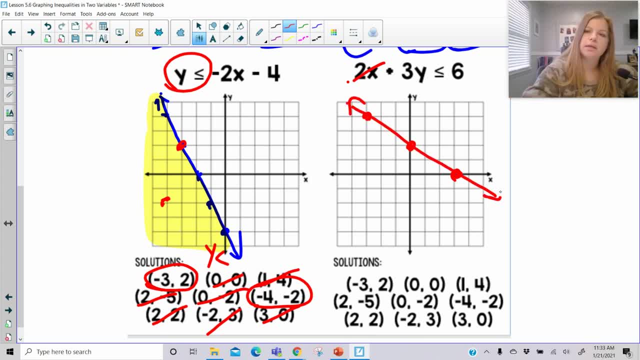 I can connect those points And then it says Y is less than or equal to. So this is where Y is less than or equal to, Equal to there, And then remember that means this is the entire side of the graph that we shade in. 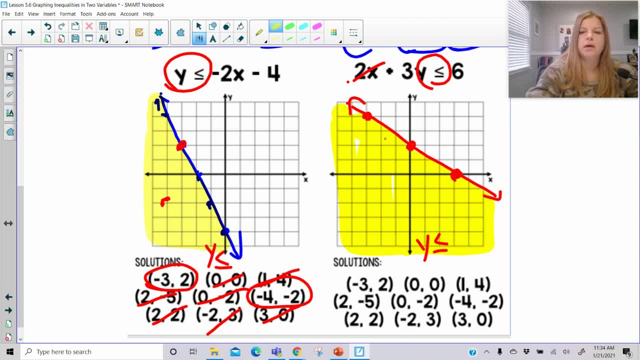 I think you get the point now about where we are shading in. So now, negative three: two is good. Zero, zero is good. One, four is not Two. negative five is definitely in there down here. Zero, negative, two is good. Negative four: negative two is good. 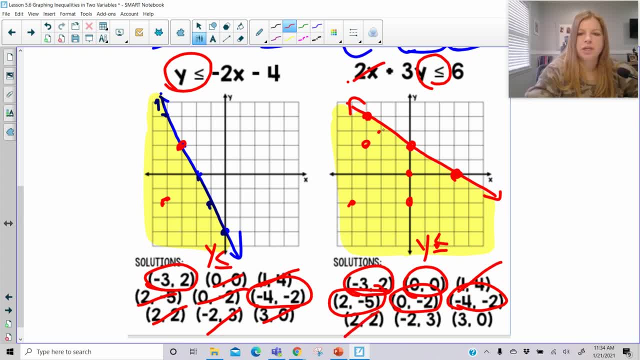 Two, two is not Negative. two, three just makes it. And then three zero is on the line, which is good. Okay, So I've got four last points, So I've got four problems here for you. Now we're going to greater than. 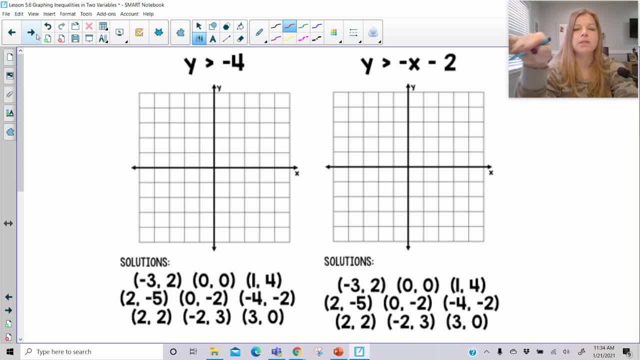 So Y is greater than negative four. So remember, if it said Y equals negative four, that would mean you would go to the Y axis at negative four, And then it's a horizontal line. So before I draw a line, remember we look at the symbol. it's greater. 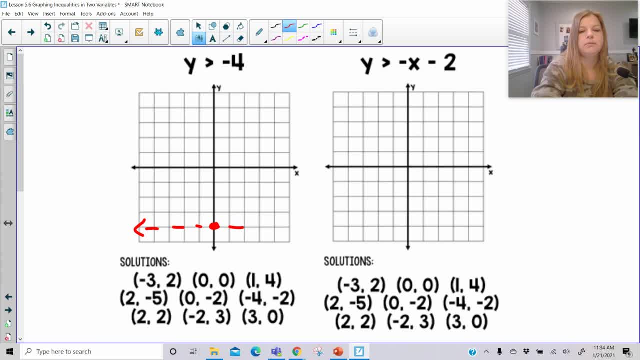 Greater means it's going to be a dashed line. And then we still take a look and say, well, where does Y get greater? Y gets greater at the top. So then this is the entire part of the graph That we shade it. 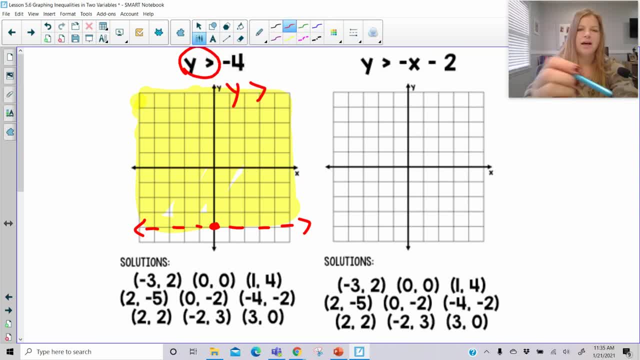 Okay, And then I'm looking at my ordered pair. So I could go through these ordered pairs really methodically, or I could just be like I'm going to look at the ordered pairs And as long as the Y value is greater than negative four, it's in the solution. 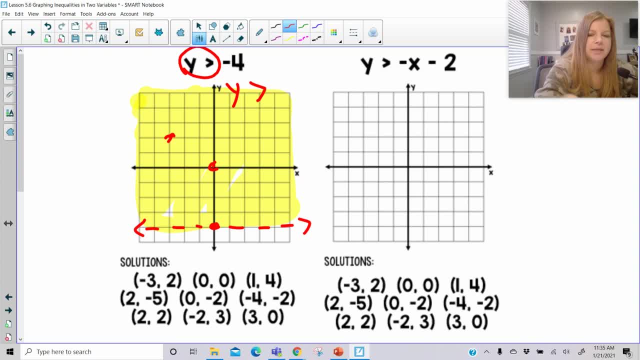 So look at this: negative three, two right Zero, zero one, four. What we actually care about are all of the ordered pairs where the Y value is greater Than negative four. So look, two negative five is down here. That's definitely not going to be it. 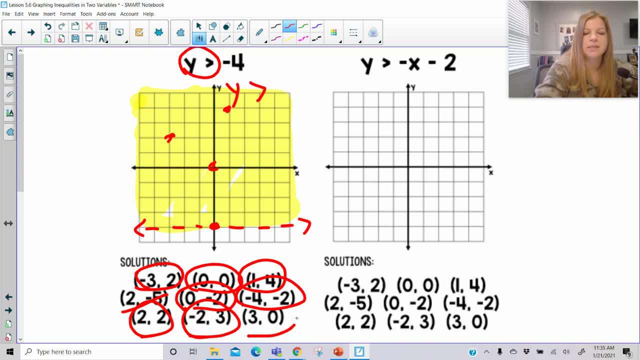 And that's actually the only ordered pair that doesn't meet the requirements. That's an easy way to do it. Y is greater than negative X minus two. So Y intercept of negative two is slope of negative one. I look at the inequality: it's greater. 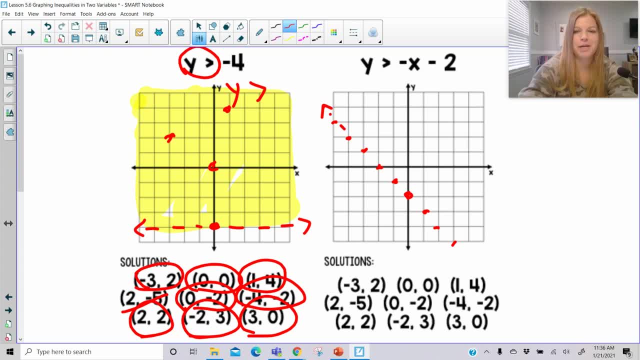 So that means it's going to be a dashed line. Sorry for me shaking my screen as I draw on it. Here is where Y gets greater. right, Y gets greater. So that means we are shading the graph on this side, Okay. 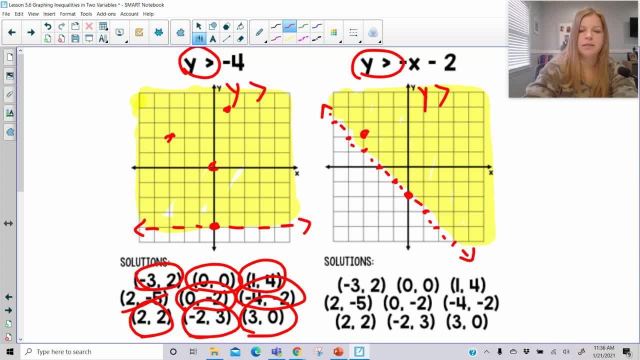 Let's take a look at the ordered pairs. So negative three: two sneaks in zero. zero is good. One four is definitely good. Two negative five is definitely right below It does not make it in zero. Negative two is on the dash line. 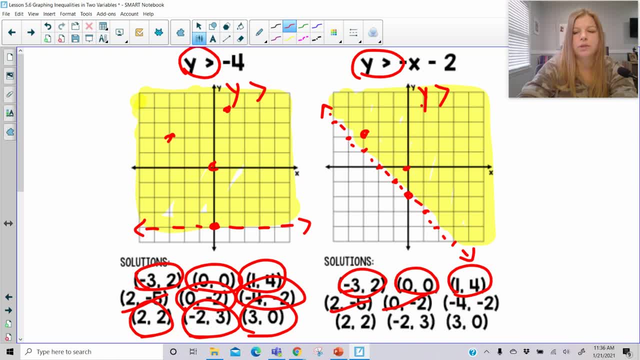 Remember, if it's on the dash line, it's not Part of the solution. negative four: two is definitely not in the shaded. two two: It definitely is up here. Negative two: three is definitely in the shaded and then three zero is definitely in the shaded. 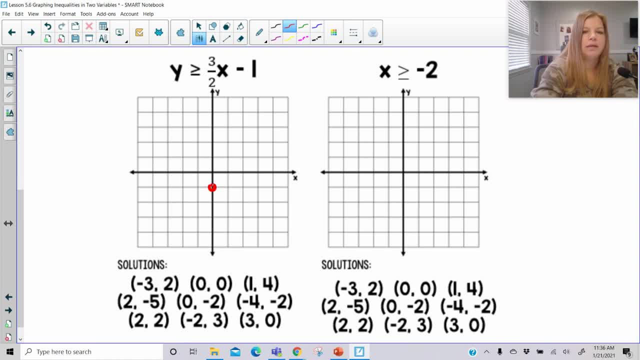 Okay, Last two problems. So Y intercept of negative one, a slope of three over two. I look at the inequality symbol. It says greater than or equal to, which we know means a solid line. It says Y is greater than. here is where the Y axis gets greater. 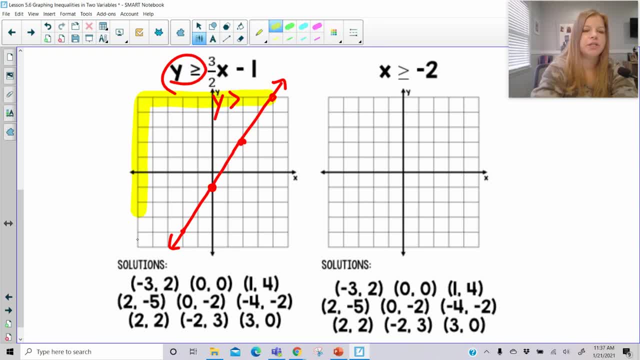 And so that's the side of the graph that we shade. Take a look at these ordered pairs now. So negative three: two is good, Zero, zero just squeaked in one. four is definitely good Two. negative five: No way Zero. negative two. 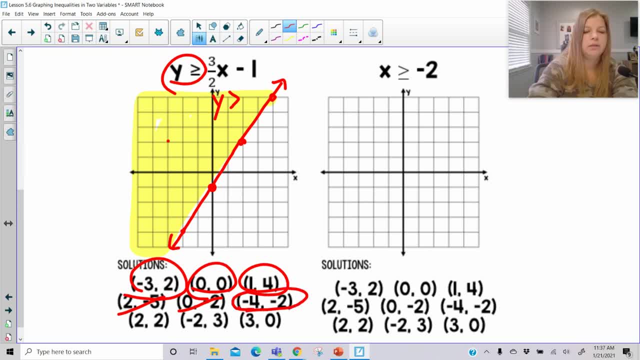 Definitely not. Negative four: Negative two is good. Two. two is right on the line, Which is good. Negative two. three is good And three, zero is not good, Definitely not there. Okay, Last one. So this one is just a slight difference, because now it's just X. 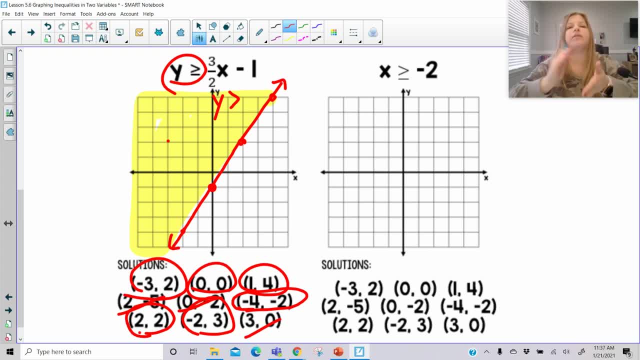 Notice there's no Y, No Y, So everything's going to revolve around the X axis for this last one. So if it said X is equal to negative two, that would mean on the X axis I would go to negative two and I would make a vertical line. 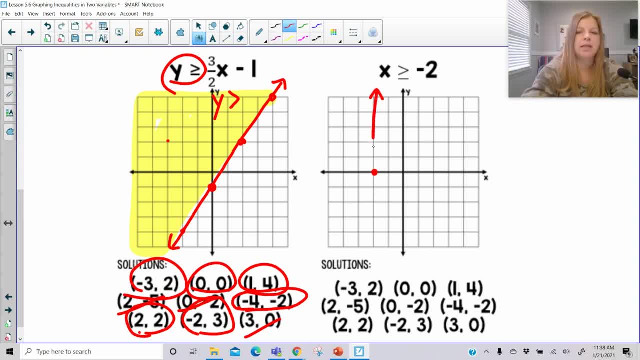 It is greater than or equal to. So that means it is going to be a solid line. And then, Okay, And then, instead of focusing on the Y axis, we focus on the X. So then I would ask you, on the X axis, where do values get greater? 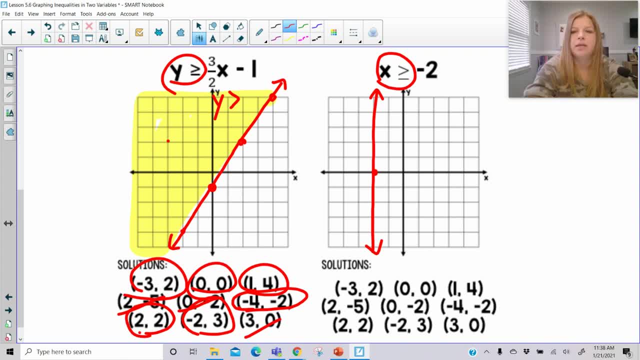 Do they get greater to the right or do they get greater to the left? This is the side where X values definitely get greater right. This is the side of the X axis where X values get less. They get smaller on that side, So that means that I would shade this entire side. 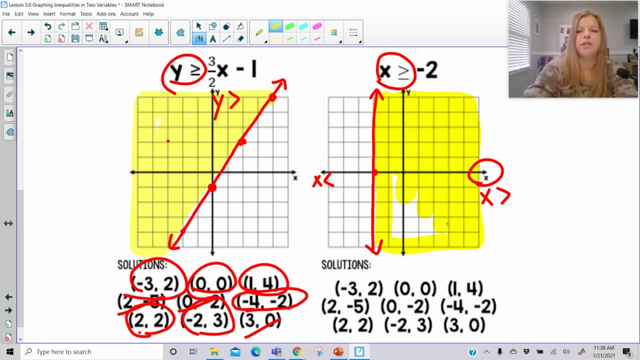 And, just like we kind of did the other trick of really just looking at the ordered pairs, As long as the X value is a number that's greater than or equal to negative two, it's part of the solution. So look: negative three two, that X value is less than negative two. 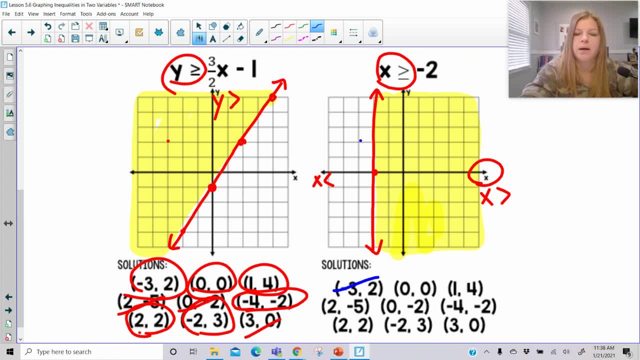 So it's definitely not there. And look where it is. It's right there, right? Zero. zero is good. One four is good. Two negative five is good. Zero negative two is good, Negative four. negative two.